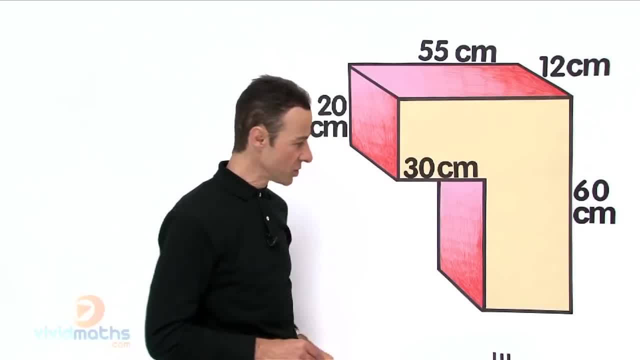 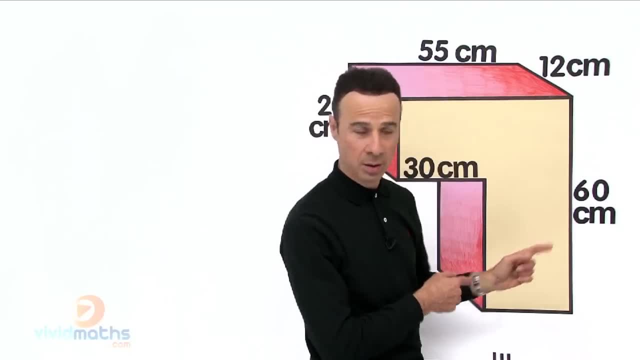 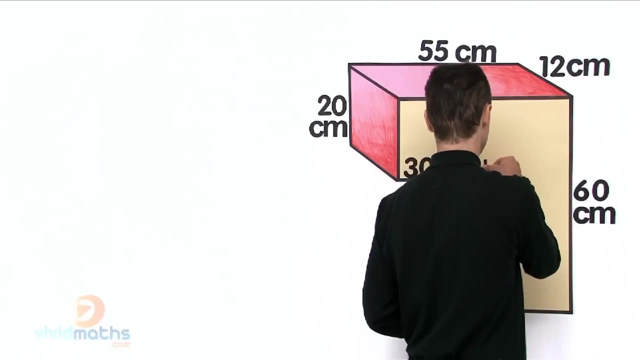 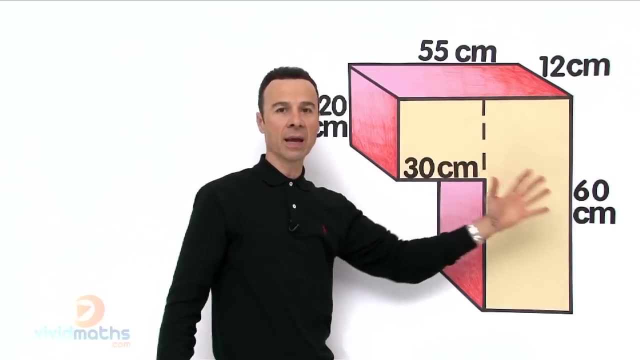 So for now, let us break it up into two areas, so allow me to make the incision. I am going to cut straight across there, so excuse my back while I make the incision. Ok, there is our incision straight across there, right? So it is area here, area there. 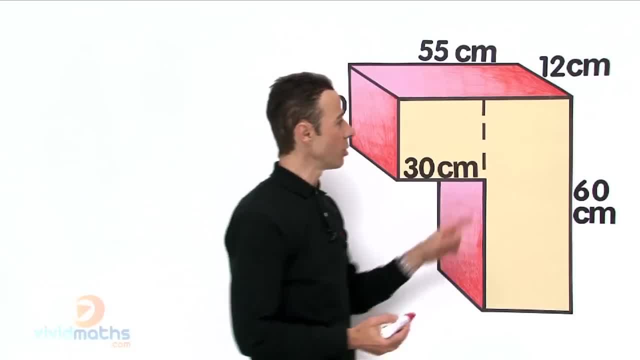 let us make up those areas, let us label them. so I suggest we call this area here right there, area one. Let us mark out those areas, let us label them. so I suggest we call this area here right there, area one. 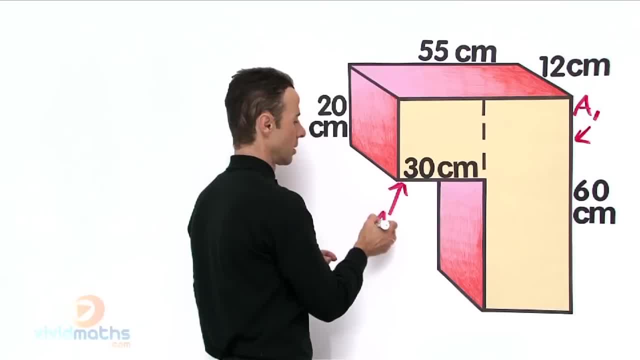 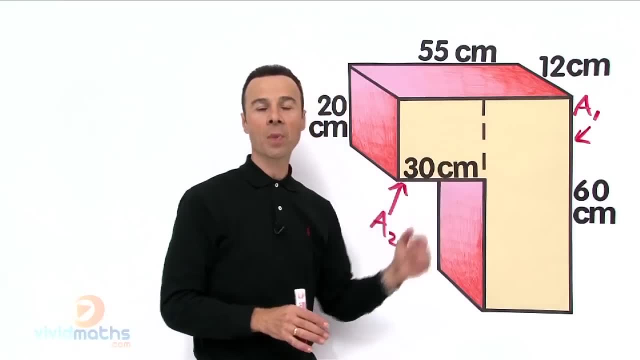 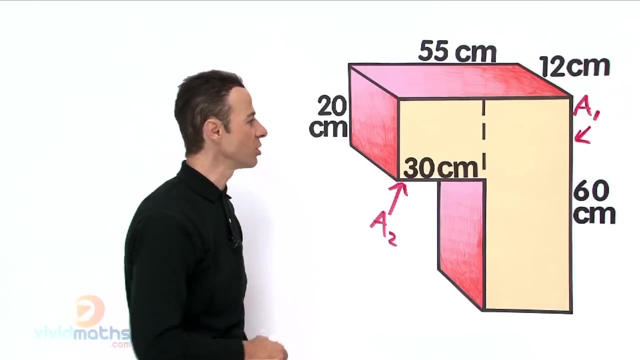 and this area here, area 2. then we combine the two areas together. area 1 plus area 2 is the total face area across there. then all we have to do is multiply by the depth, of course, in order to get the volume. Now let us go back to what we have. now we have got these two areas, so let us actually 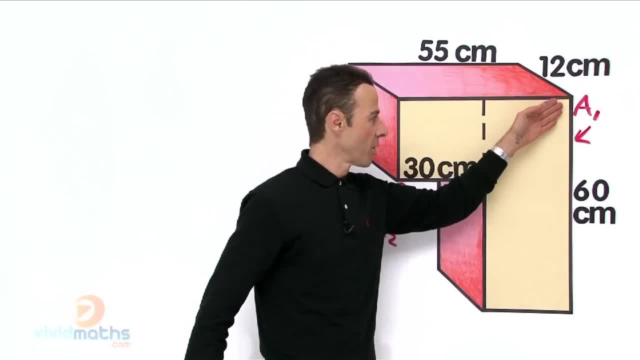 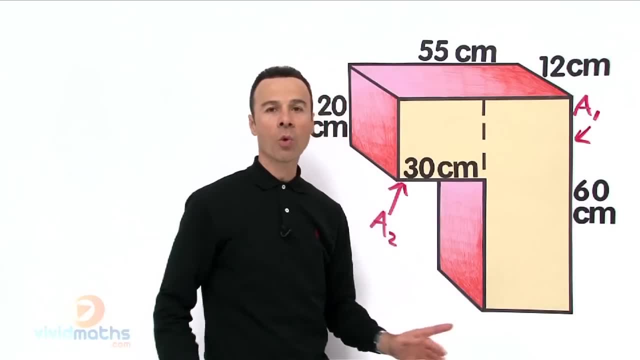 work out area 1. so area 1 will simply be this times that, but we do not have this missing length there, remember I talked about that earlier? so how do we find that missing length? Well, here is a trick and a tactic, a strategy, if you like, that can help you deduce and determine. 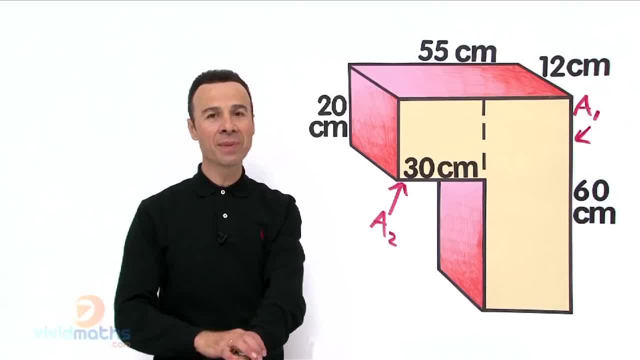 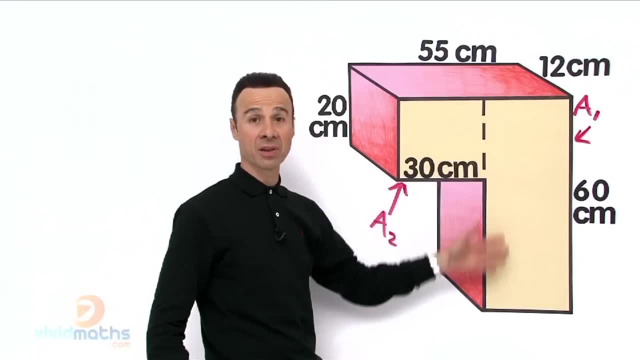 what these guys are. How do we do this? Well, the trick is this- and I am sure many teachers do not actually state this, but a few would know this: The thing is, if you are looking for a missing length in a complex shape like this, you always 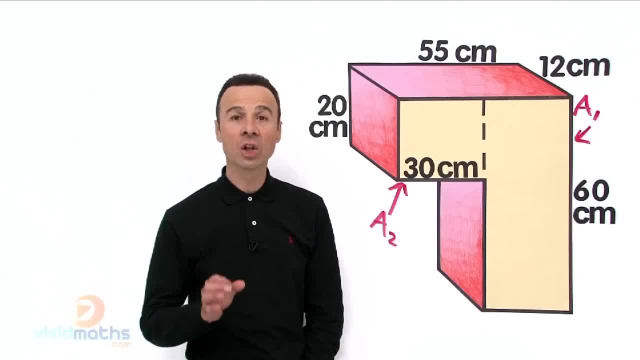 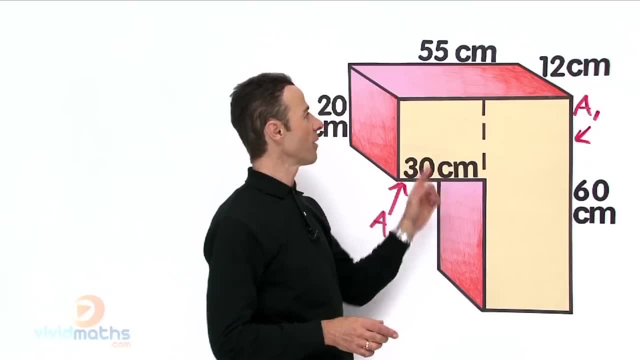 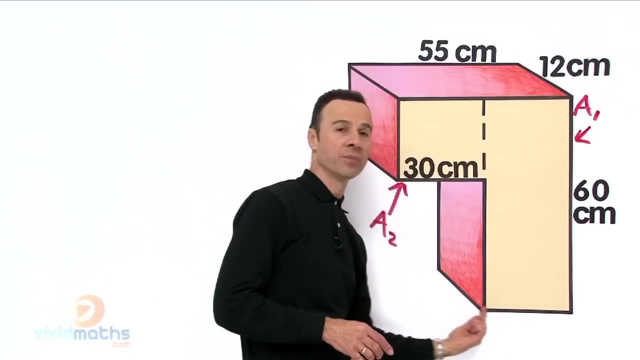 search and look for parallel lines. Parallel lines are the clues. So let us have a look at what parallel lines are Parallel lines we have here. I will show you what I mean. well, we have a parallel line here and a parallel line here, and the line we are looking for is parallel to that notice. 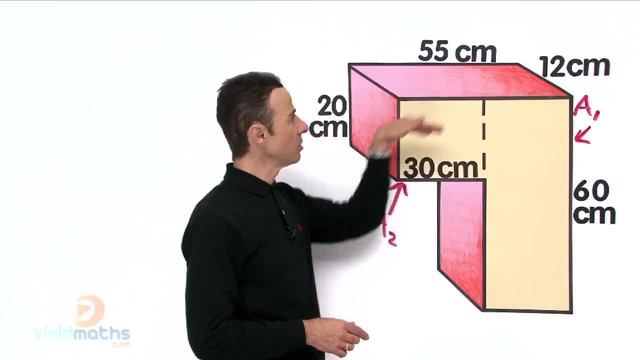 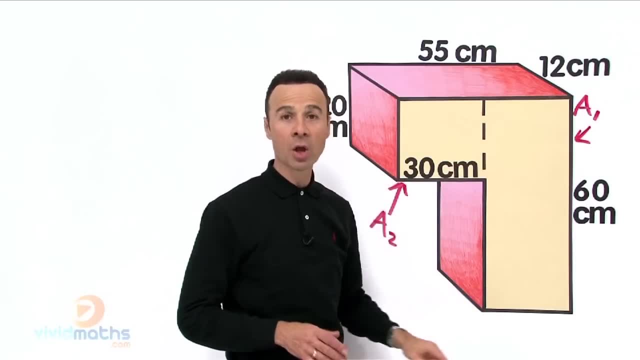 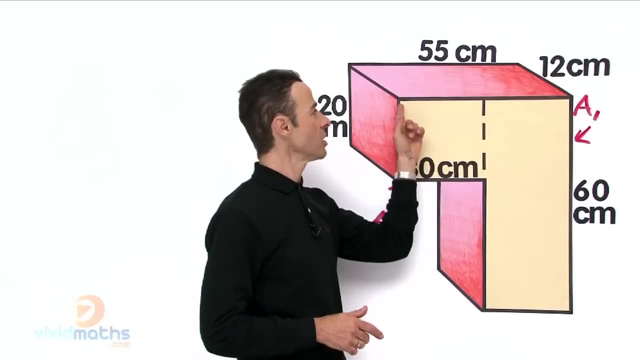 that that is horizontal, horizontal, horizontal. they all go together. Now, by using all those horizontal lines, which are all parallel, we can actually deduce what this is here, right? So let us see how we are going to work this out. So this line along here, we know is 55.. 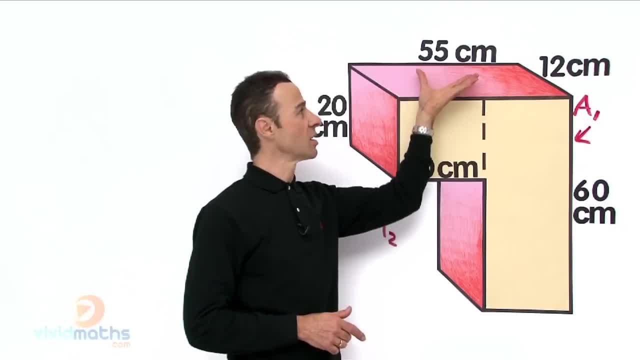 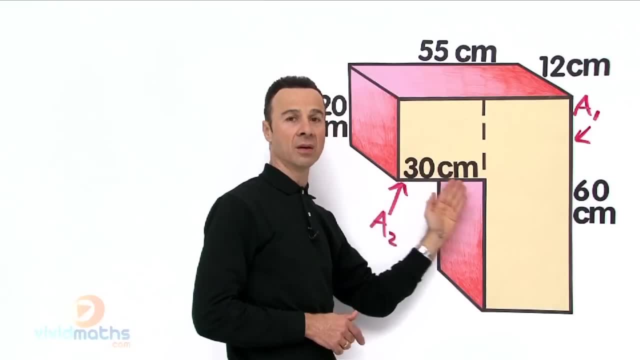 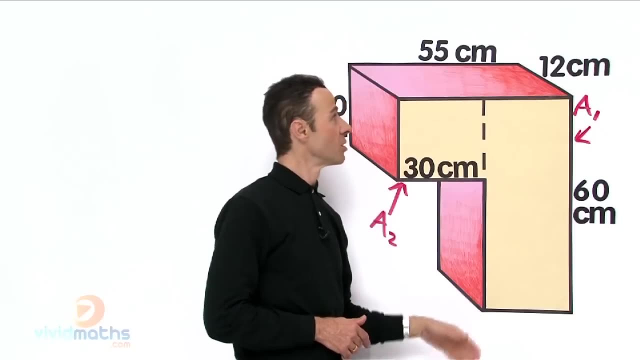 Because back here it says 55. ok, so let us transfer that down here. So it is 55 along here. take away 30 over here will leave us the gap here or the gap here, it is the same because they are all horizontal. yeah, 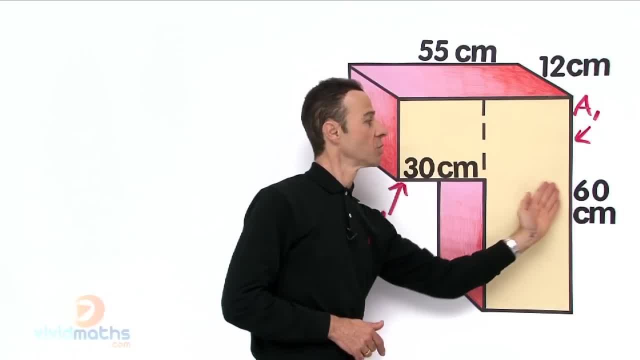 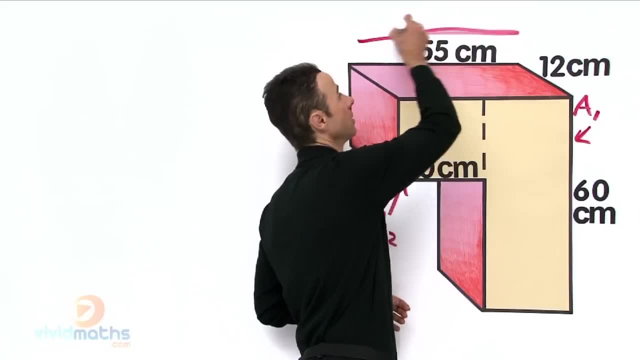 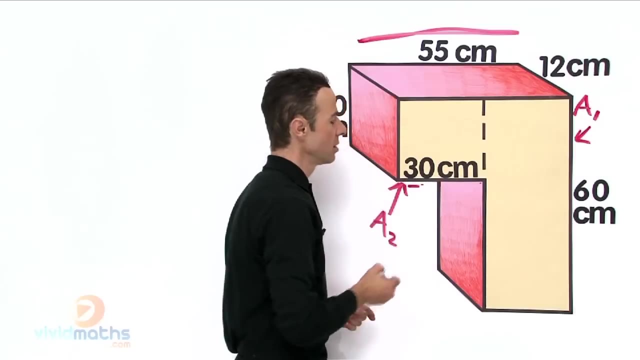 So 55 minus 30 gives us 25. that will be 25 there. So let me mark it out for you one more time: The distance across here, Take away the distance across here, across there, all the way across there, that distance. 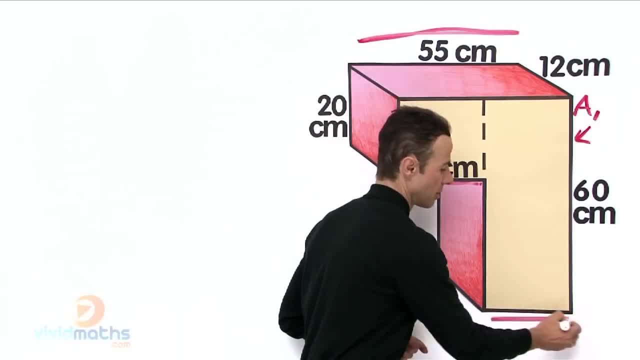 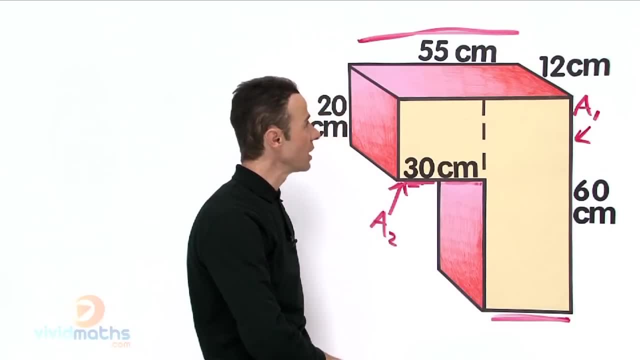 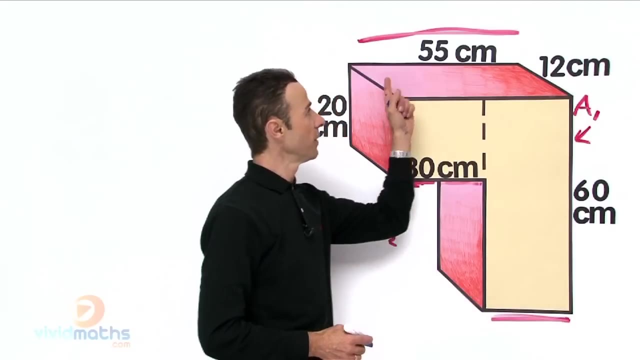 there, that minus that will give us that there or that. it is the same. So let us do that now, let us work them out. So for area 1, right over here, we need to find this length: here: 55 minus 30 gives us 25.. 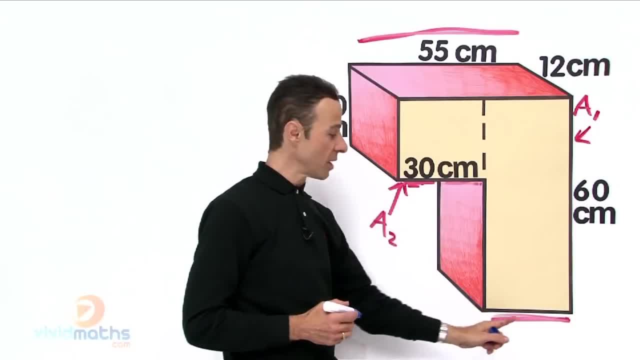 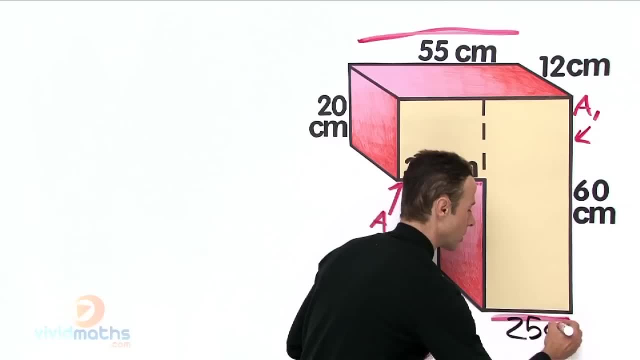 55 minus 30 gives us 25.. 55 minus 30 gives us 25.. So that means this missing length there is 25.. Can I write that in? Let me write that in There is our 25, which means this is also 25 across there. 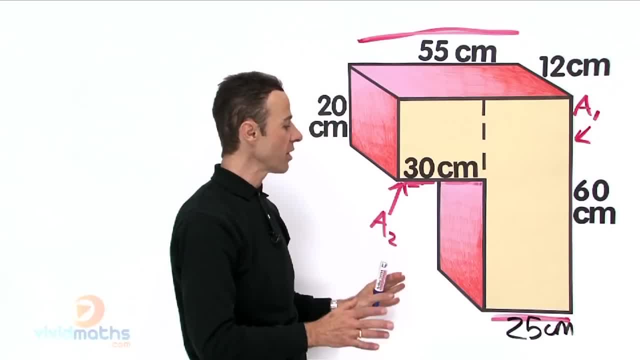 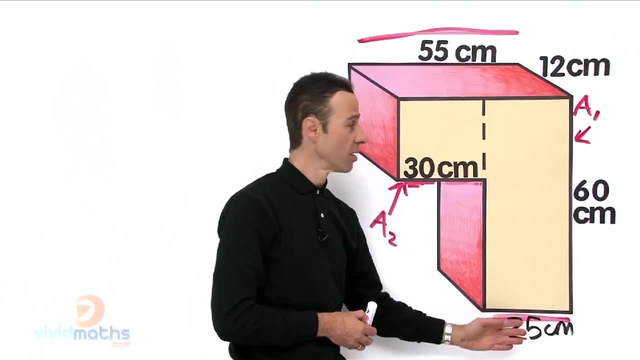 Ok, we have established. that make sense. Yep, Alright, now that we know that all we need to do to find this area is what Length times breadth we have the missing length, so 60 times 25. so let us do that. So for area 1.. 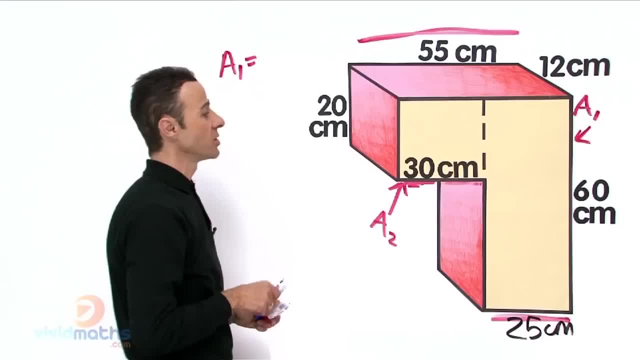 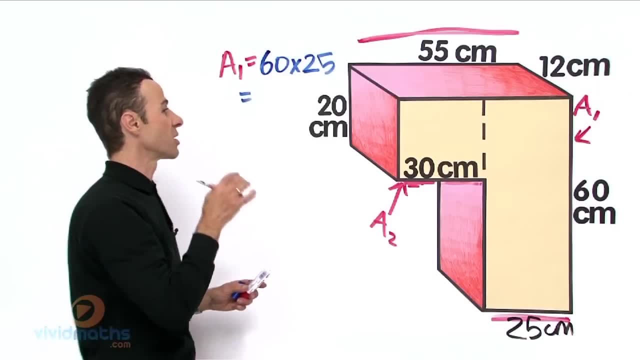 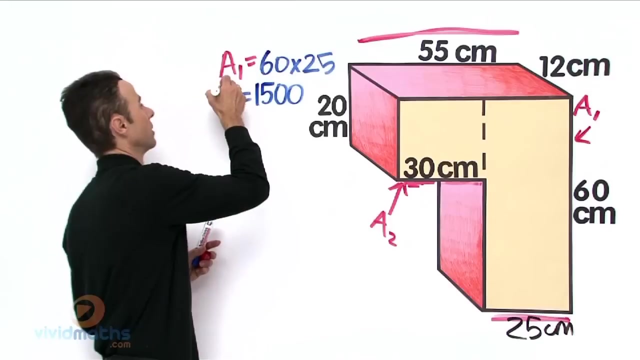 60 times 25, which equals on the calculator: 60 times 25 is a grand total of 1500, so that is going to give us 1500.. Ok, that is area 1.. Area 1 is 1500 centimeters. 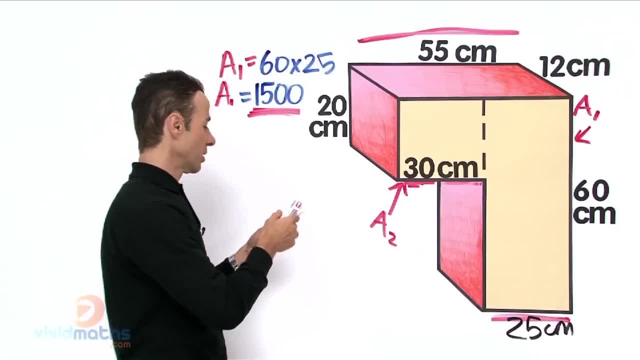 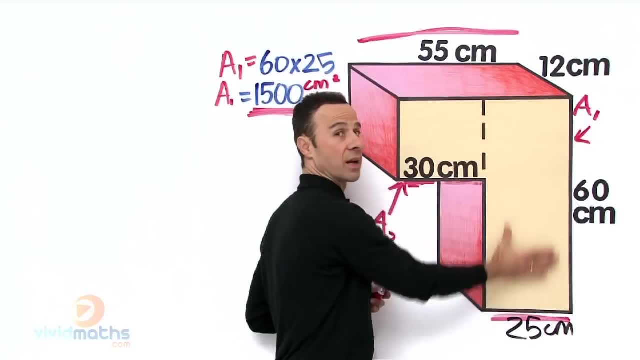 Ok, Centimeters squared because it is in the units of. let me write it down: centimeters squared because that is an area. so that is area 1, all the way across there. can you see that? Alright, now let us work out for area 2, which is this one in there. yeah, 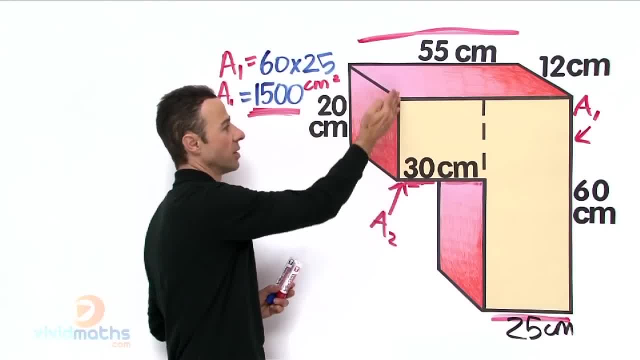 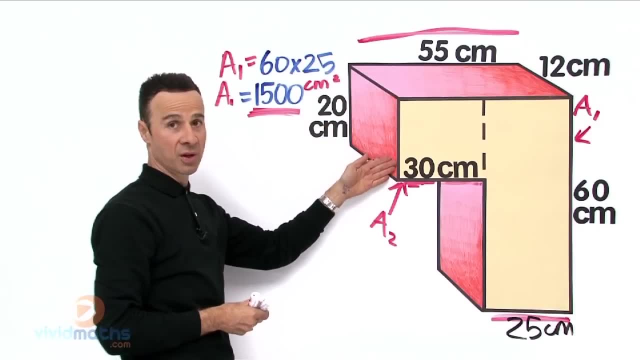 So that is going to be 30 times the height. now that height is vertical and that is also the same there. can you see how they are the same? If that is 30 here, that means this is equivalent 30 there also. they are both parallel and 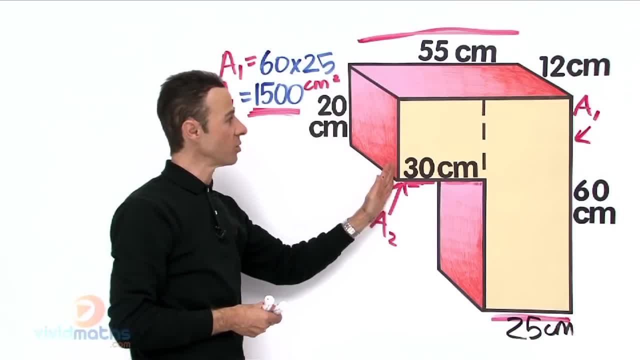 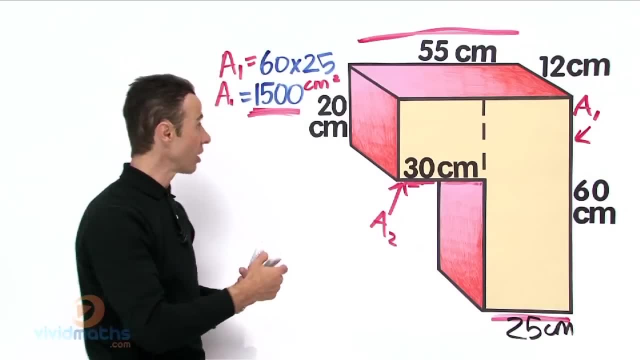 they are both vertical. yeah, So that is 20.. So that is 20 also, So we can mark that out as 20,. yeah, So 20 times 30 gives us a grand total of. let us work that out. 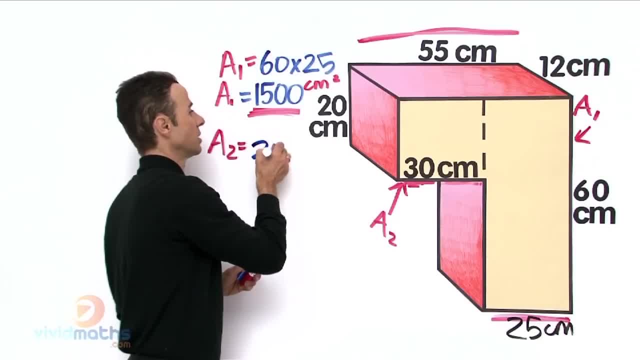 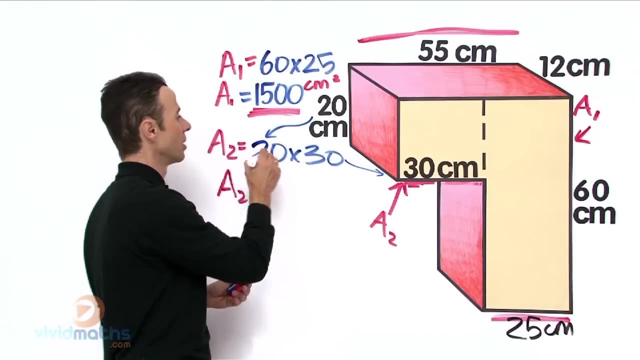 Area 1 equals 20 times 30, because that 20 is transferred there. there is that 20, right. That goes there and that goes there. Ok, 20 times 30 on our calculator for area 2 equals that is going to be 600, isn't it? 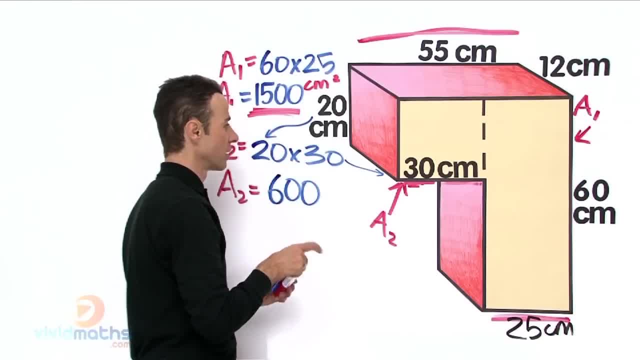 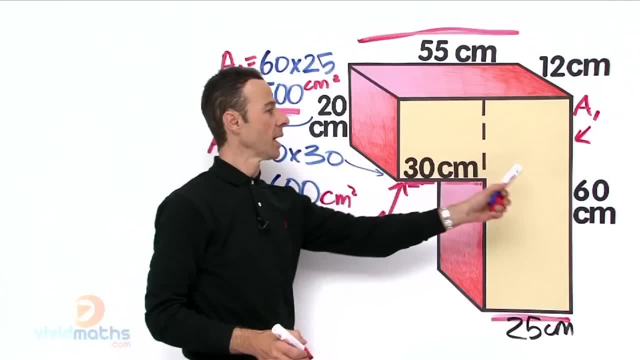 And that is also centimeters squared. Alright, There is our area 2.. Ok, Area 2.. Area 2 here, area 1 there. Now, all we need to do is take the two areas, combine them, add them together. let us do. 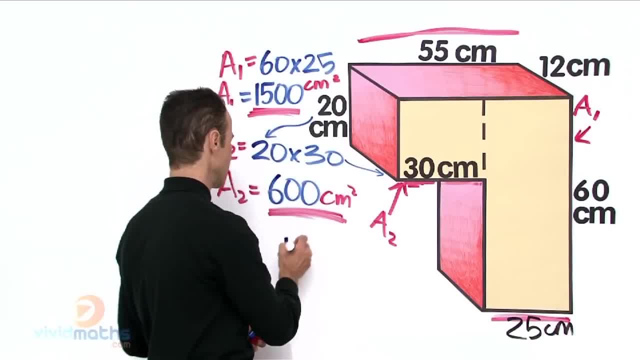 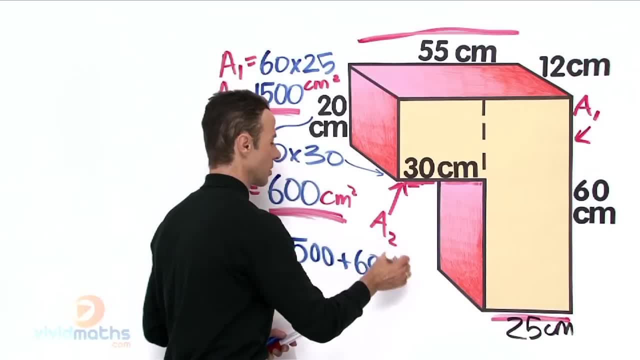 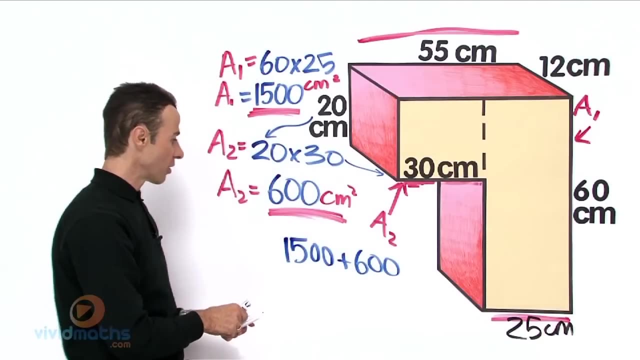 that. So we are going to have 1500 from up there, area 1 plus area 2, 600 and that is going to give us a grand total of what all that faces in beige the total area there. So that is going to give us a grand total of area of the face equals area 2 plus area. 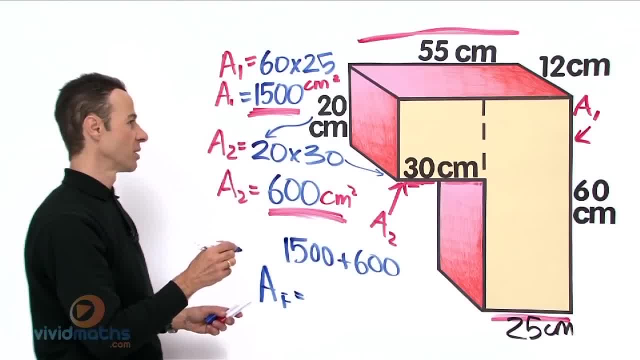 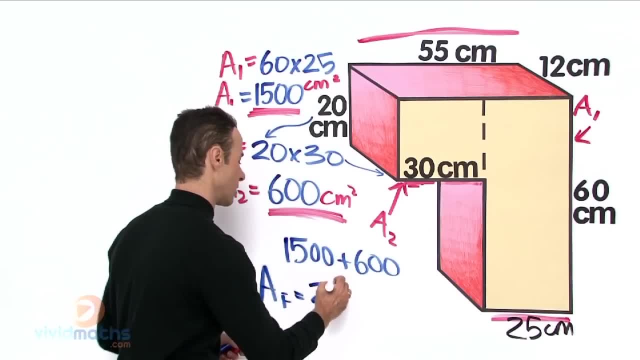 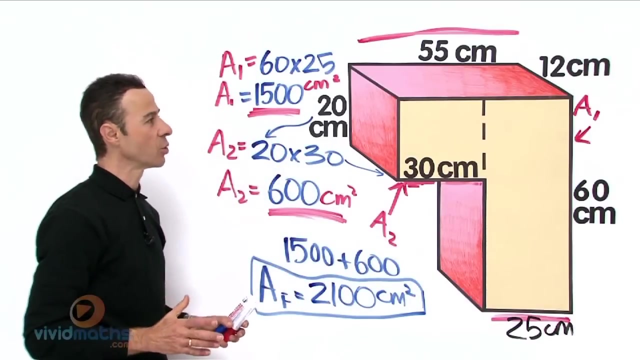 2 equals 1500 plus 600 is going to give us grand total of 2100, and that is centimeters squared. So there is our area of the face all the way across there. Ok, we got the area of the face. now all we need to do is actually work out the volume. 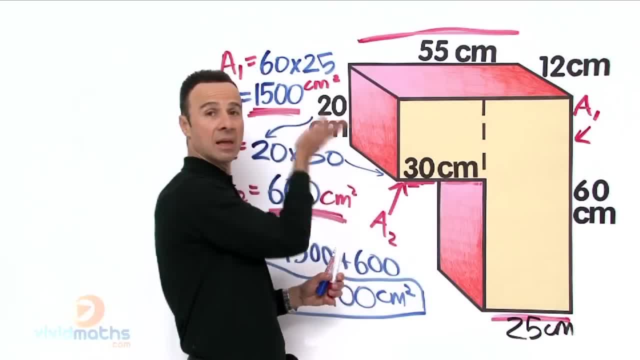 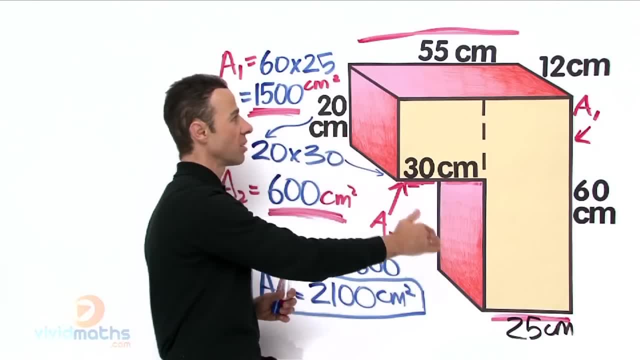 and in order to work out the volume, it is obviously face times depth. Ok, Now what is the depth here? Can we see the depth written? Which number gives us the clue? The depth is all these lines that go like this diagonally: 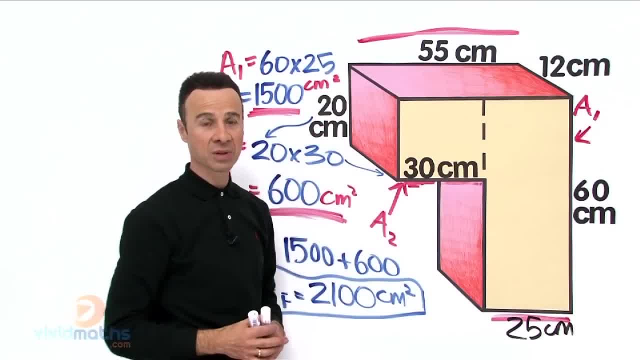 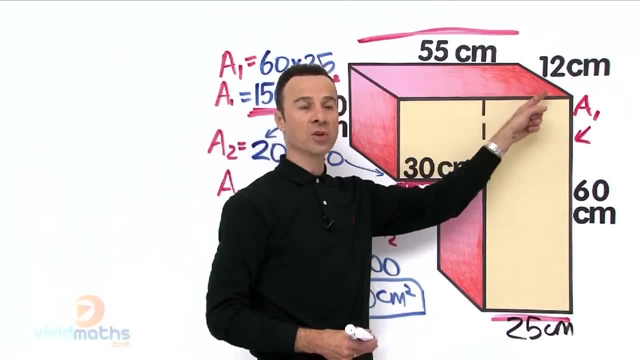 See them. All of them are the actual depth. So it is not here, it is not there. it is not there, it is actually there. See that. That is 12, which means this is 12,, 12,, 12,. they are all 12,, they are all parallel, remember.